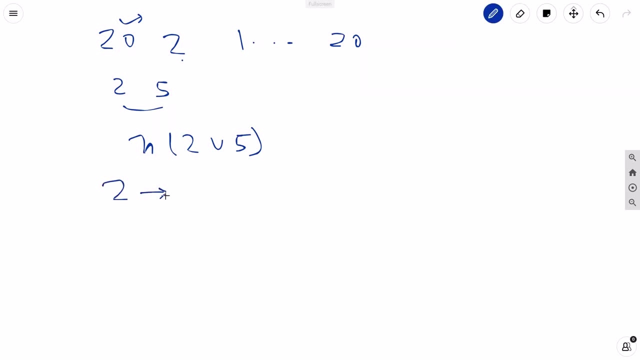 okay, so let's see how many numbers are multiples of two. so for two, two, four, six, eight, ten, twelve, fourteen, sixteen, eighteen and twenty, these are multiples four, and this is the second one. so the second one is a five. so here it's five. five, ten, fifteen and twenty are its multiple. okay, so now, if you want to get, 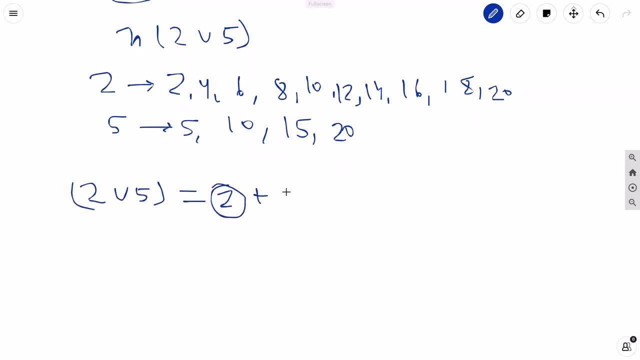 this two union, five, then what we have to do, you can just add this: two and five, okay, but when we are just adding this, uh, two and five, 20 is added twice. so these duplicates we need to remove. so these are getting duplicated because this 10 is a multiple of 5 as well, and 2 as well. so what we will do, we will remove duplicate. 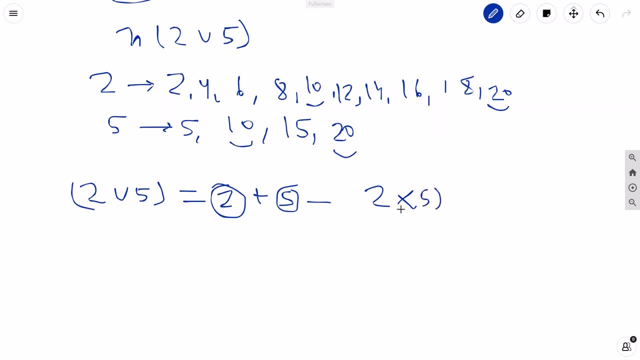 which are multiples of remove numbers which are multiples of 2 and 5. so like this we will do which is like 10. so for 2 we are having 10, for 5 we are having 4 multiples and for 10 we are having 2 multiples. so total we will have 12. 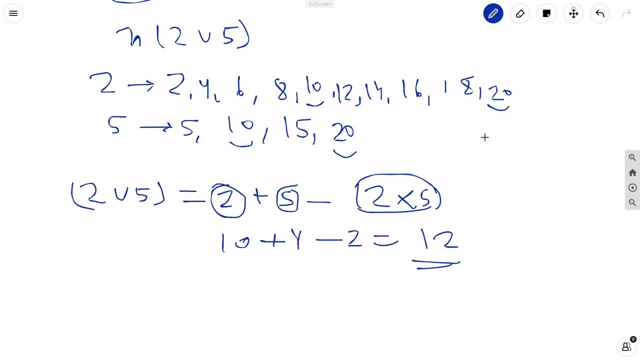 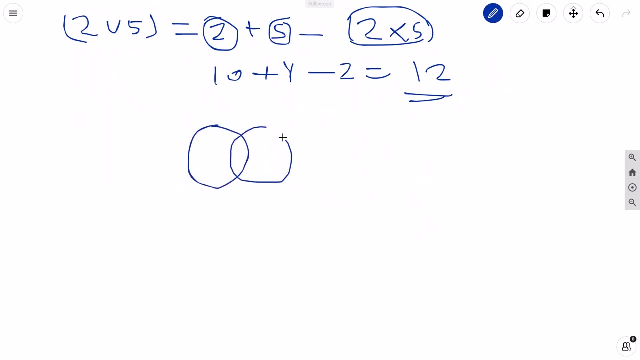 so this is how we can get answer for simple test case. now, in our case, number of prime numbers can be up to 20, so let's see how we can solve with that. okay, but before that let's see this venn diagram. so we are having these two sets, a and b. so if you want to get 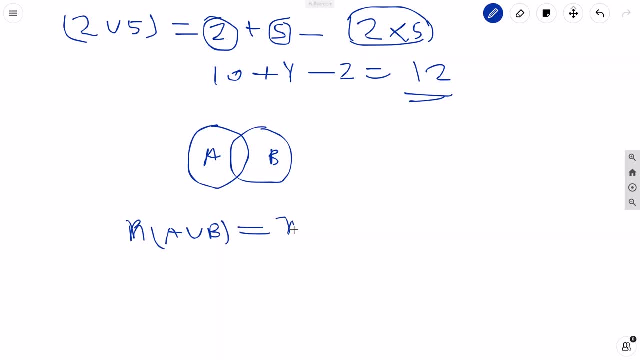 number of elements in a union b, then what we can do is we can select n, a number of elements in a in set a and we can add this. so this we can do like n, a, and then we can do this and b. and now, since this is getting duplicated, 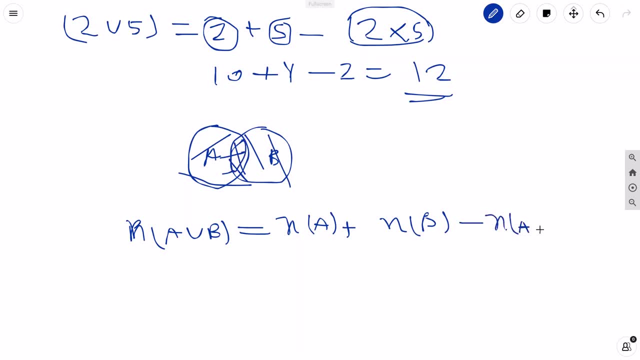 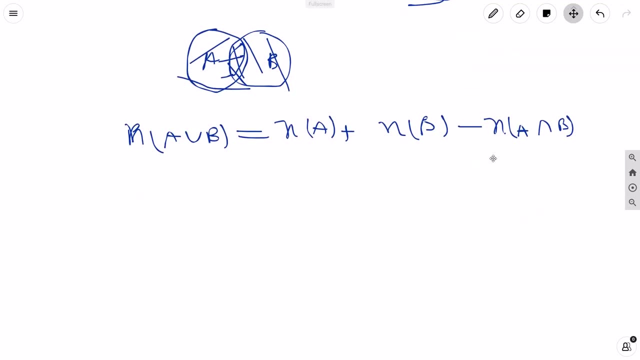 so we can do n, a and then k, and we can add n and b, and now, since this is getting duplicated, so so we can remove this one, one copy of it we can remove. so this we can do like that, okay. so now let's see how we can. 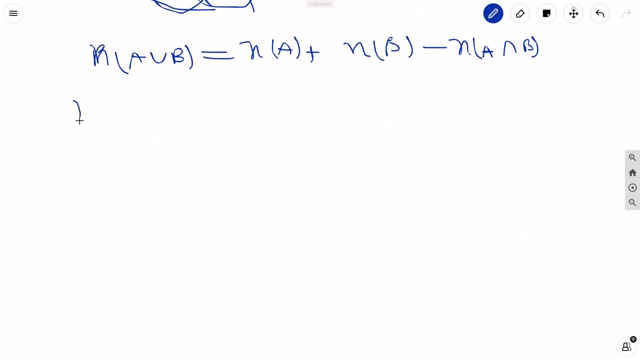 generalize this so that we can have something like this: n a union, b union, like that for multiples sets, because that is what we want, because we will have more than one prime number, more than two prime numbers. so p1 union, p2 and p3 up to pk. that is what we want. so this we can do using inclusion. 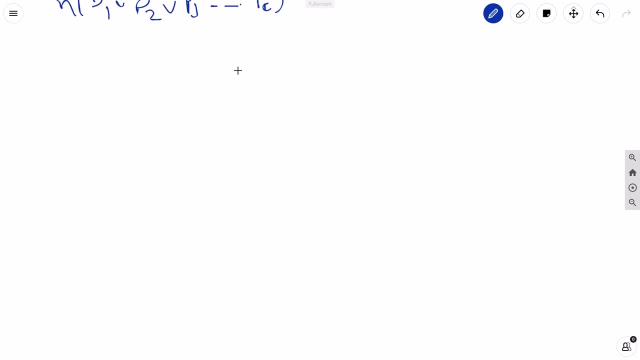 exclusion principles. so let's see how we can do that. okay, so i will just write formula. so if you are having k sets, distinct sets, then for them to get this union. what we can do, we can just take some of all of ai, some of all of ai. 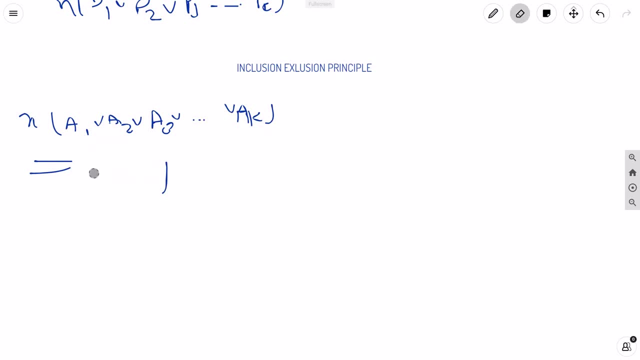 some of all of ai. i will write it again. okay, so we can take some of all of ai. i equal to one to n, so this means you and a1 plus an, a2 plus anything like that. then we can take all of pairs from this and. 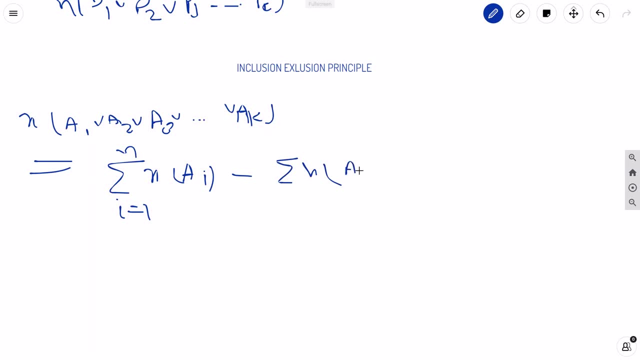 subtract it. so like that, ai intersection h we can do. then we can add all triplets in there, okay and uh, like that we have to do. at the end we will have minus one to power k, plus one n and the other results we get this minus half squared, so that one is like that. 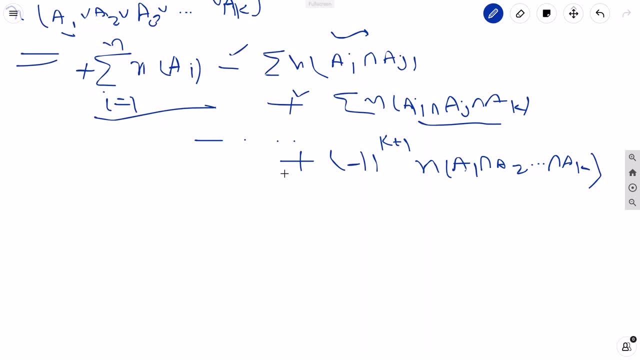 minus Letterer. Now you can see the variation. this is the difference between numbers. so it is mid, which is ages plus here and three in the class. then we can talk about some of the variables here and not just one. then we are talking om them, then we are picking two of them or from all the sets and we are summing them, then we are picking three and then we are picking four, like place pointsUL, gravities laws. 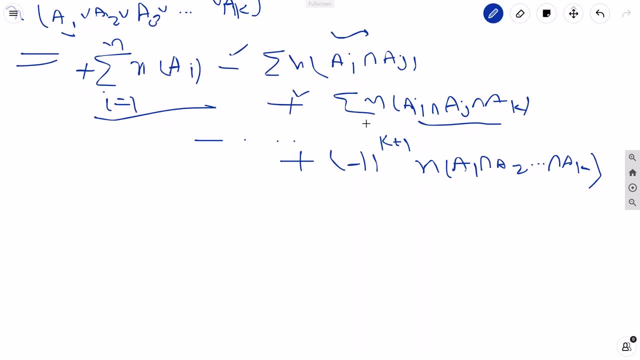 go on. okay, and one thing is like: if number of sets are odd, then uh, even so, if number of sets are even, then this will be minus negative. if it it is odd, then it will be positive. so now let's write this: pa1, union a2, union a3, using this inclusion, exclusion principle. 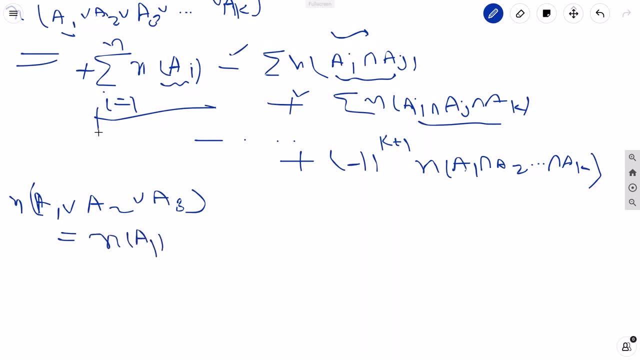 so this will be an a1 from this first line. so this we can write just something more. then we have to pick two of them and subtract. so we will pick even an a2 first, then a23, and then a1 and a3 and then this third, since these are negative. so it will be composite. 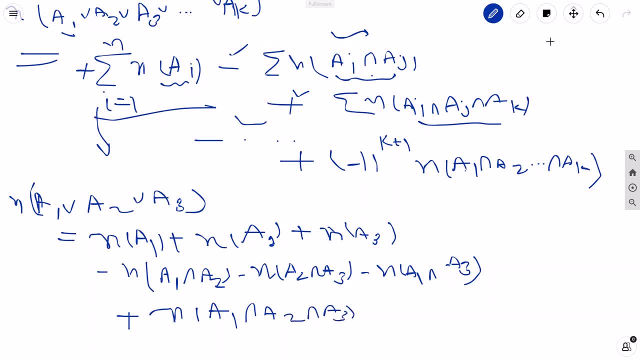 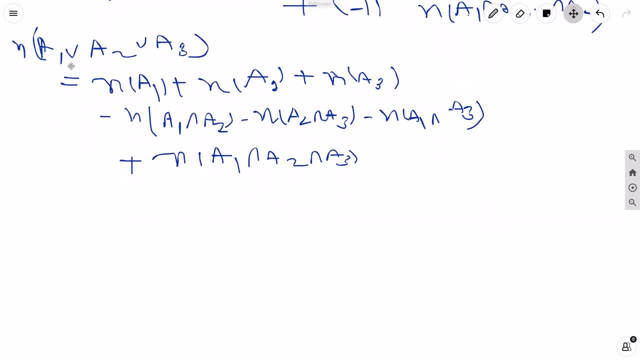 so this a, a2, even a2, a3 we can add. okay, so this is how we can get this a1 union, a2 and a3, like that. okay so, and now we're going to let's see how we can solve our problem using this. 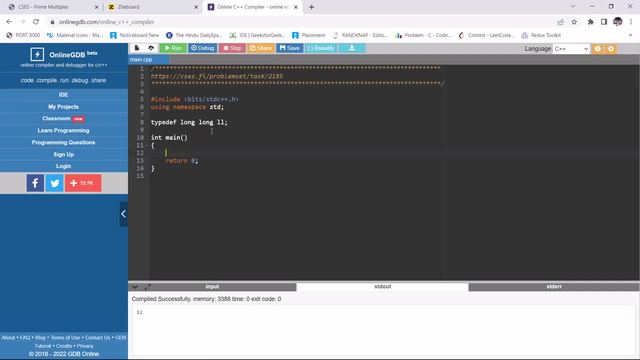 okay, so first okay. so here i am going to use a long long because our numbers are in 10 to 18 range. so tick and okay, i will take input and then i will take a primary in which i will input all of those prime numbers. if we need this, all the things in particular are well sever. okay, then here you have this. 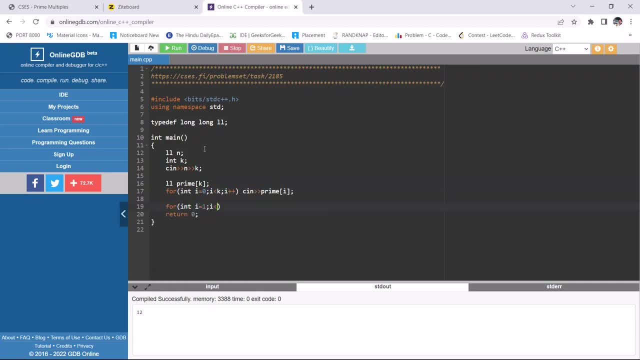 threeے here. that's the one a. you just add. that would be just like this. so so that's the solution that we can get. you could take every combination possible from this son asd, and if you do that, you just, and then what we are doing now is we will just do like this. 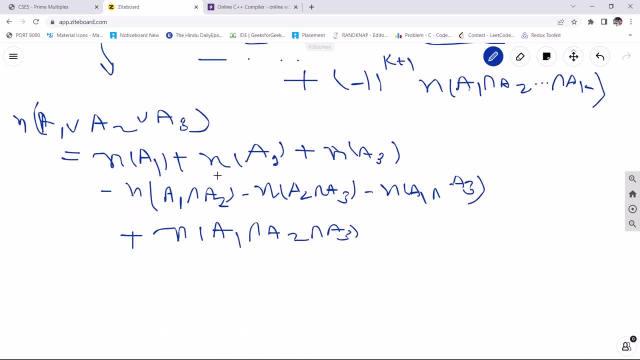 okay, then what i will do? i will just like this, okay, and this i will explain you, okay. so so here, if you see in this example only a1, union, a2 and a3, we are taking every combination possible from these two sets. so we are taking when only one is there, a1, a2, a3- when only two are there, 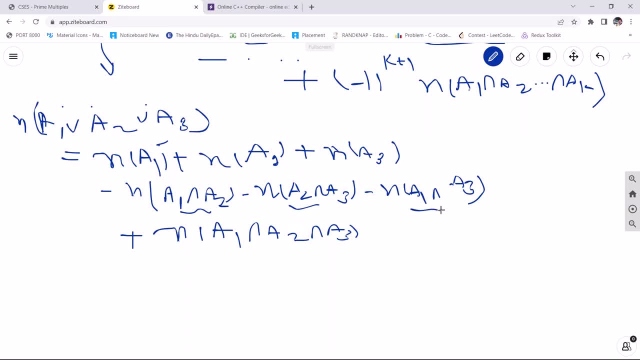 so a1, a2, a2, a3, a1, a3, like that, and when all of them are there, okay, and we are not taking counting that set in which no one is there, so empty set, we are not considering so total. we are having this two to power, k minus one sets here, okay. so here in code also we will do the same thing. so we need. 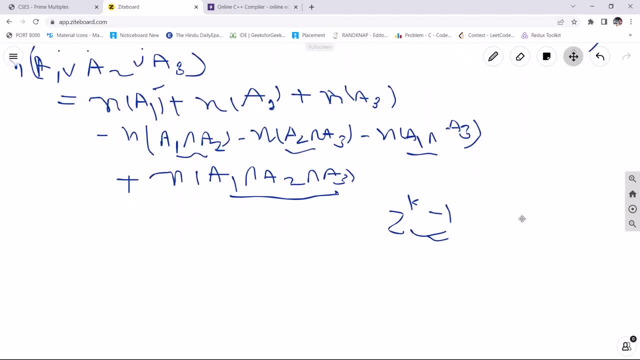 to consider every combination. yes, every combination we have to consider. so the way we are going to handle this in code is so we can take k bits and these bits are will be corresponding to integer value. so we can say 0, 1, so, and up to true to power k minus one there will be. so here all bits will be one. 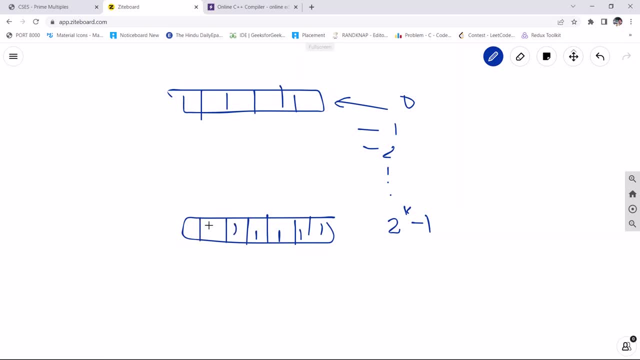 and in starting for zero, all bits are zero and we are assuming they are just k bits. okay, so if you take just, uh, someone from middle so say: for this, this bit is one, zero, one one and zero like that. so what this means is so if this bit is set here, then this means so. 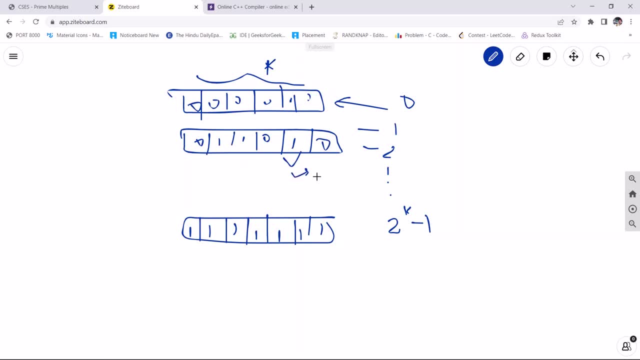 corresponding to this position in our primary, so that prime number will be there in the number we are picking. okay, and when this is zero, that means that prime number is not there in the number we are picking, so for which we want to calculate multiples. similarly for this also, and when we 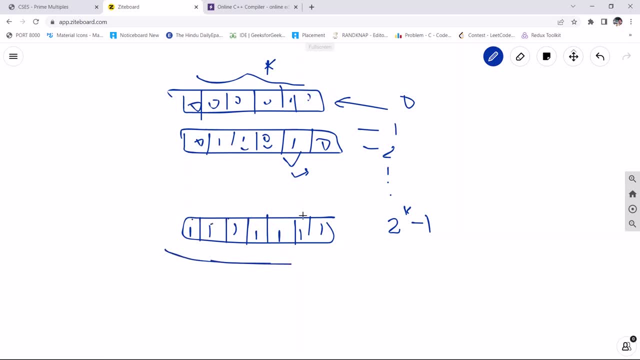 are at this end. so this means every prime number is there in the number for which we are interested in finding multiples. okay, now how do we actually find out number of multiples for a given number? so from one to n, we have to find out. so if you want to find out for, let's say, like two, so what? 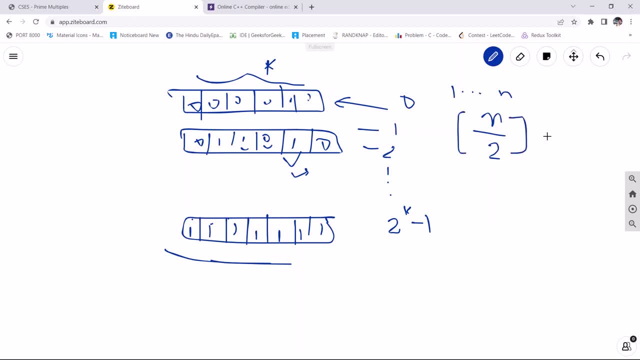 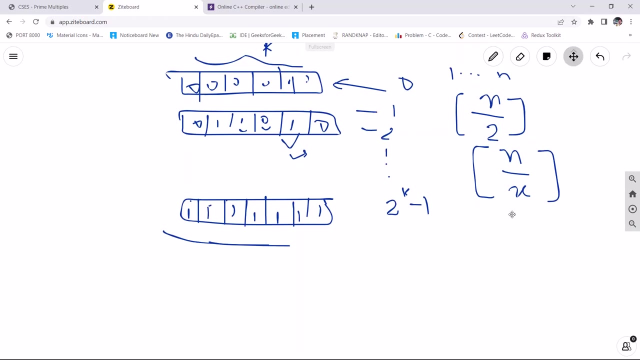 we can do: just do n by two and take integer part of that. similarly, if we are just having an x number. so what we can do, just take integer part of this n by x and we will get number of its multiples, which we are actually interested in. so okay, now one more thing: this x here will be product of 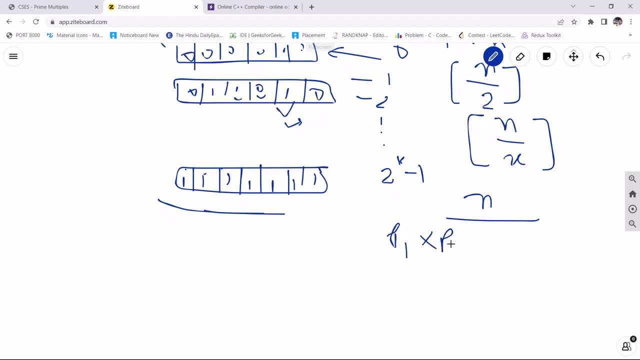 this prime numbers. so it will like this p1 into say like: if it is not present, so p3, into p4, into say like by five, six are not present, so p7. now this p1, p2 are up to 10 to power 18.. so if you multiply them, 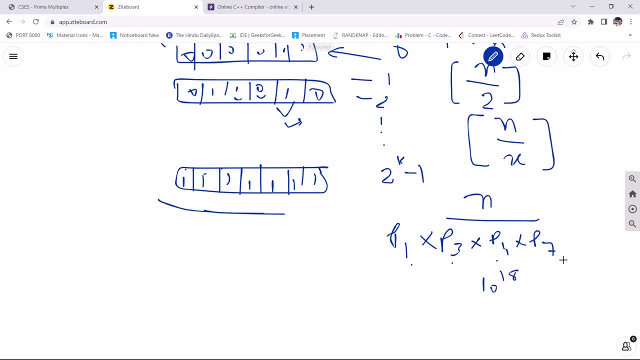 and then uh, just divide this n by that, so then it will overflow. so what instead we will do? we will uh divide this n by p1 first, okay. then we will divide this uh by p3, then we will divide 8 by p4, and then y, p7, like that we will do, and then we will get number of multiples for this. 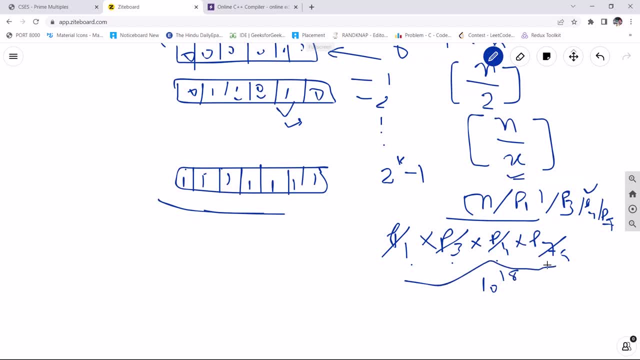 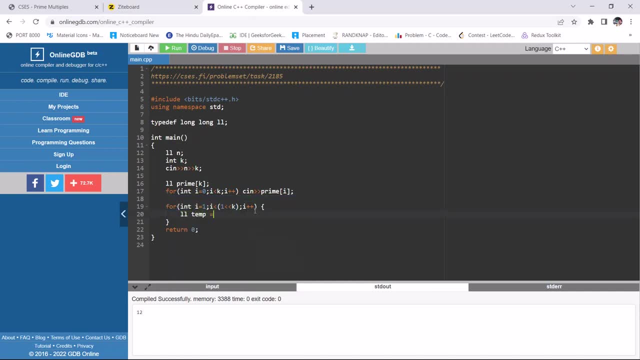 number x or this number. okay, so now let's again go to the code. okay, so i will take an temperable. this will be number of multiples, so initially it will just one n, then for each bit in i we will traverse, so there will be k bit in which we are interested. so then i will take 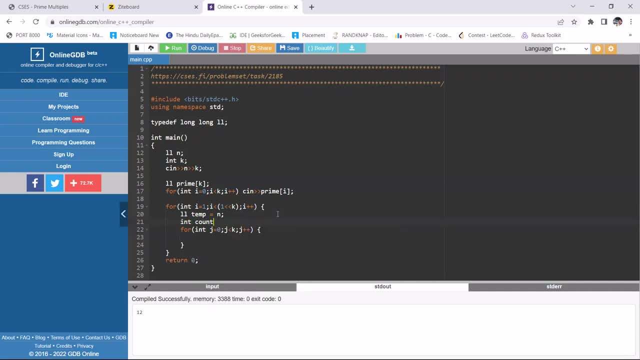 a variable and i will store in, in which i will store number of set bits. so i will just count set bits or you can say count sets also and this will tell number of sets. so initially zero. so then i will see, check okay, if in that i that bit is there. so if it is there that means we can increase our concepts by one. 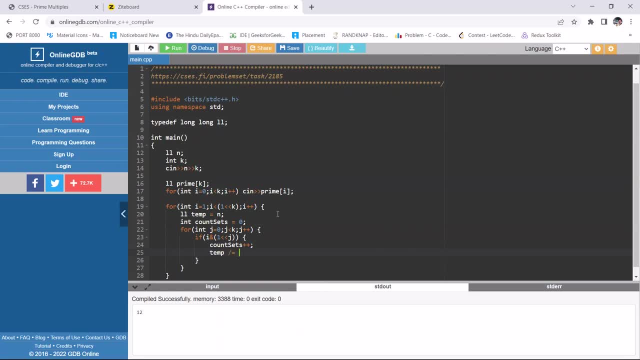 and we can divide this temp by this prime j, because since j th bit is there, that means this prime j is there. so to calculate number, we can just divide this temp, which is initially n, by prime j. okay, now here what we can do. you can check if that concept is odd. so if it is odd, then we can add inside our